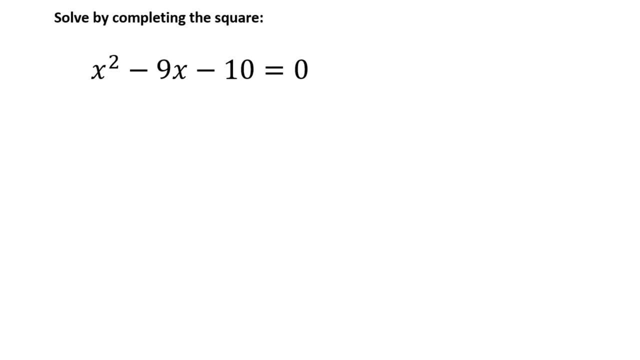 Now, guys, please bear with me here. Your teacher might do completing the square in a different way to what I do. You do not have to follow your teacher's way, and you also do not have to follow my way. You must choose whichever way you are comfortable with. Just make sure that you're. 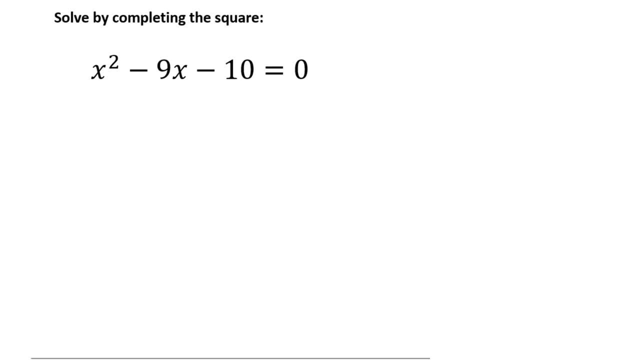 getting to the same answer because, as I said, there are different ways. So what I would do, and what a lot of students do, is they would take the 10 over first. then we can open up a bracket like that, and then we're going to take x minus. 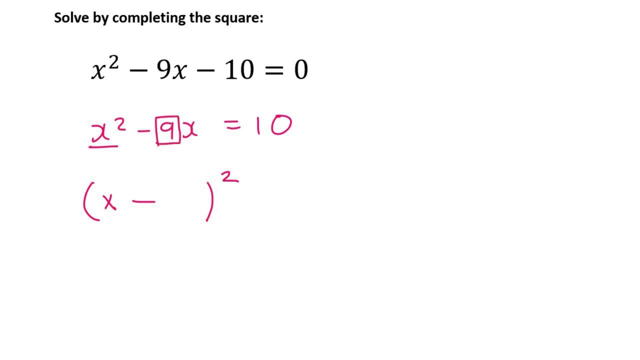 now you must always do this: divide this number by 2, so that's going to be 9 divided by 2.. Now you might have another step in between. I know some students do do it like that, but I'm just using the shorter method and 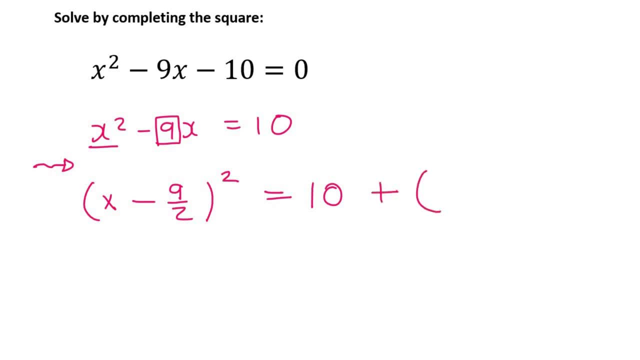 so then on the right hand side, you're going to say 10, then you're going to say plus, then you're going to put this number into a bracket squared. If you can remember this pattern, you can do really well with completing of the square. Let's go through that carefully. What did we do? So what? 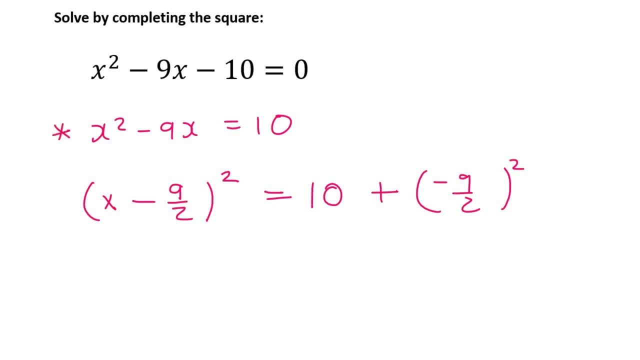 I did first was I took the 10 over. that was this step here. Then I open up a bracket and I put a square and then I take this number and this number divided by 2.. Then I put the 10 over here, because that 10 was already there, And then I add whatever this number is in. 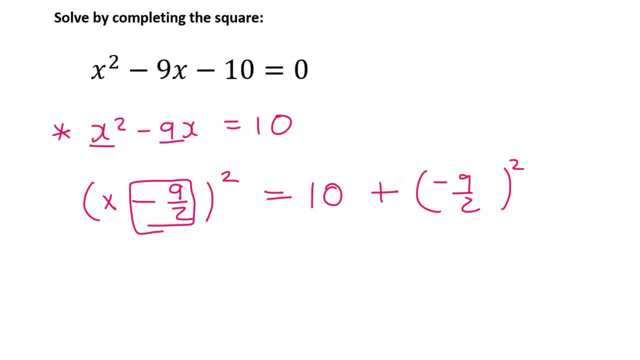 a bracket squared. That is all that you need to know for completing the square. The next part is very easy. So, and- and bear with me guys- we're going to do a couple of these questions. So if you still struggling a bit with these, try a few more examples and then you'll start to see the pattern. 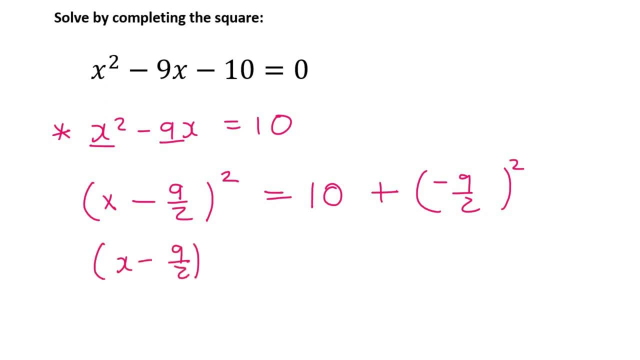 so now what we do is we say x minus 9 over 2, squared, then this number on the right. you just type that all in the calculator using the brackets- wherever you see brackets- and it's going to give you 30.25. what you now do is to get rid of the square. you're going to square root both sides.